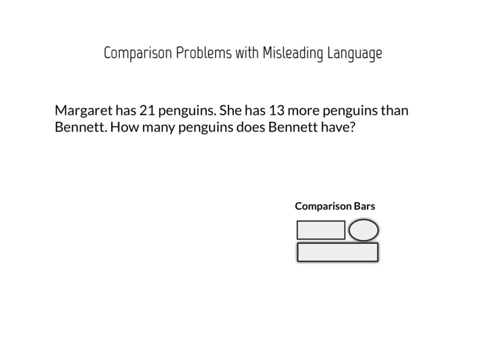 comparison bars. we're going to have to have the smaller box for Bennett and the larger box for Margaret. So I'm going to write Bennett's name here and then I'll write Margaret's name for the larger box. Okay, and if I look back at, 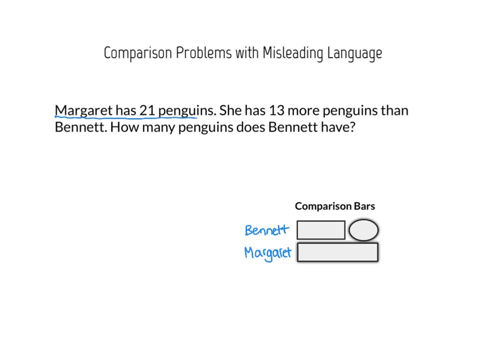 the problem. let's see what information we know. Margaret has 21 penguins, so I can put that in a larger box, and we're trying to find out how many penguins Bennett has, so that would be in the smaller box. 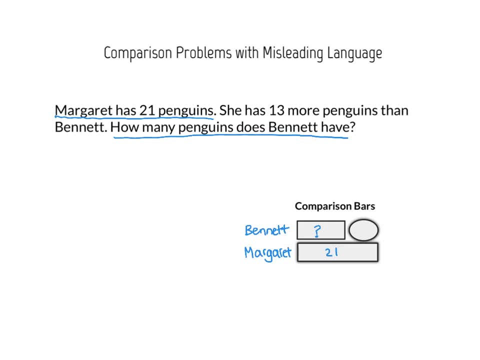 And it says that Margaret has 13 more penguins than Bennett. so that would be our difference. So whenever a math mountain- I mean not a math mountain- whenever our comparison bars are filled out like this, we know that the larger box, the larger rectangle can be used to subtract the difference to get the 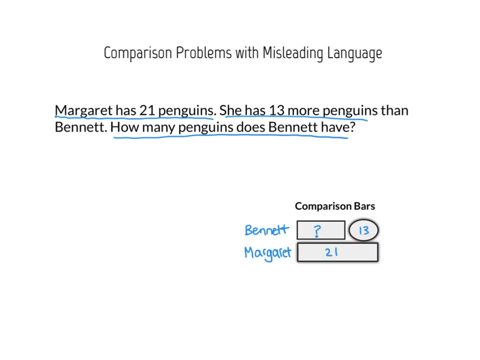 smaller one. So our equation to solve this would just be 21 minus 13,, and that would give us our answer for Bennett, because Margaret has more than Bennett. so we just have to subtract the difference. So I can't subtract 3 from 1, so I'm going to have to ungroup the 2, and that'll give me 10. 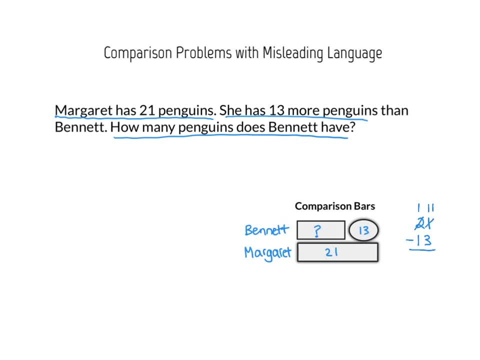 ones. so instead of having 1, 1, I now have 11.. 11 minus 3 is 8, 1 minus 1 is 0. So I got an answer of 8 penguins for Bennett, and that makes sense, because 8 is less. 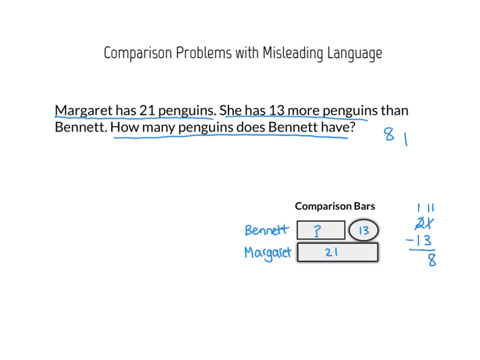 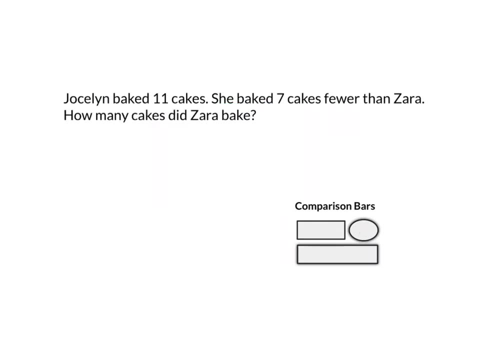 than 21.. Margaret has more than Bennett, so 8 penguins. Okay, let's try this one. Jocelyn baked 11 cakes. She baked 7 cakes, fewer than Zara. How many cakes did Zara bake? So we have to figure out what are. 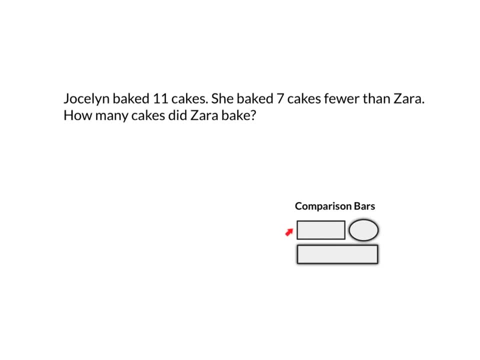 we going to write in our comparison bar Who has the smaller amount and who has the larger amount. It says that Jocelyn baked 11 cakes. She baked seven cakes fewer than Zara, So it sounds like Jocelyn baked a smaller. 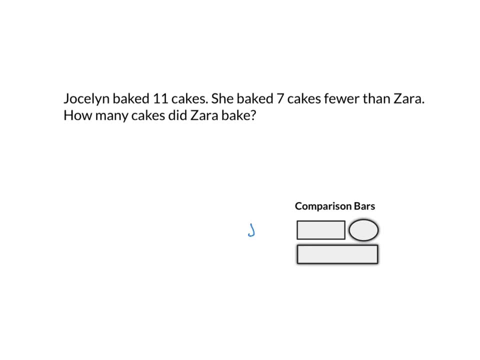 amount. So she's going to get the smaller rectangle. So I'm gonna write Jocelyn's name here and I'm gonna write Zara's name here. Now let's see what are we trying to find out in this problem. Well, it says: how many cakes did Zara bake? So 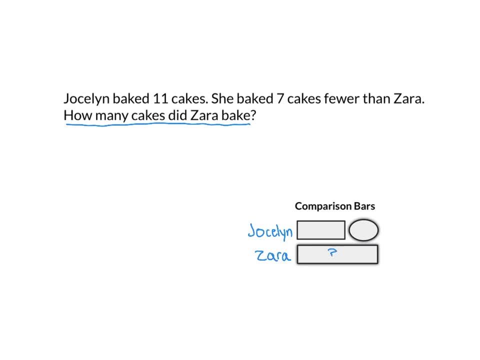 that is going to be our question mark. We want to know how many Zara baked. And what do we know? We know Jocelyn baked 11. So we have that information, We can put it in our rectangle. And she baked seven fewer than Zara. So that's our difference. 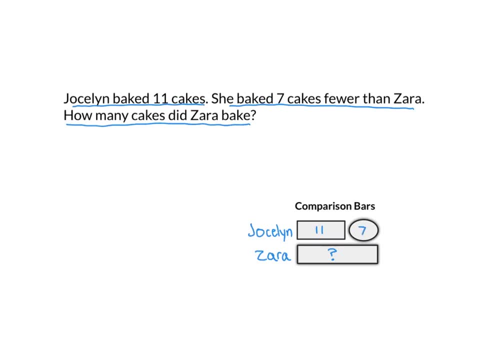 Now, when we go to solve this problem, whatever you have in your top rectangle, and the difference is always going to add up to the bottom one. So this is a very easy problem to solve. We just have to add together our 11 and our 7. 1 plus. 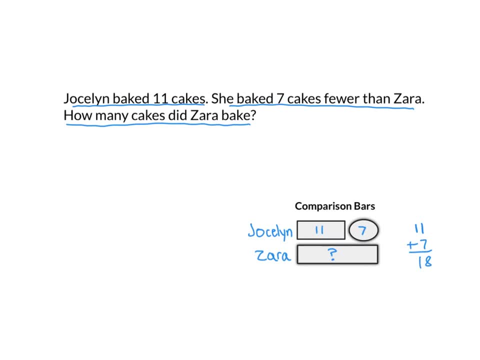 7 is 8.. 1 plus nothing is 1.. Now let's see if this makes sense. Let's go back to the problem. Jocelyn baked 11 cakes. It's 7 fewer than what Zara baked, Is 11, 7. 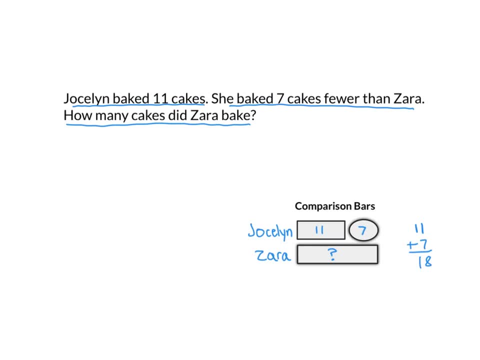 fewer than 18? It is So that would work. So Zara baked 18 cakes. Here's another one. The teacher handed out 16 books. There were 22 students in the class. How many students didn't get books? 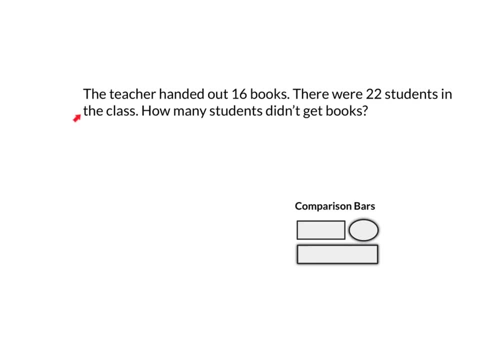 Now this problem is interesting because it doesn't use any of the words like more or fewer. but we can still solve it because these comparison bars will still come in handy. We just have to think about which information is the smaller amount and which is the larger amount. So the teacher has 16 books and there's 22. 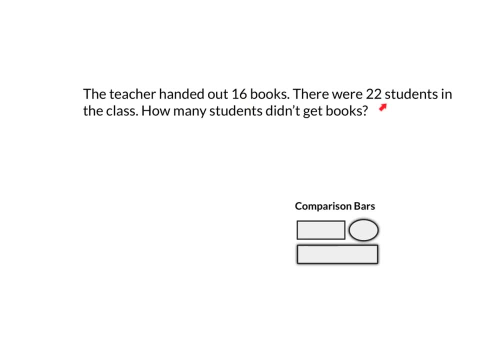 students. so it looks like there's a fewer number of books and a larger number of students. 1 is 42.. 2 is 34.. can write that down: books gets the smaller amount and students gets the larger amount, and we know the total number of books. the total number of books is 16.. 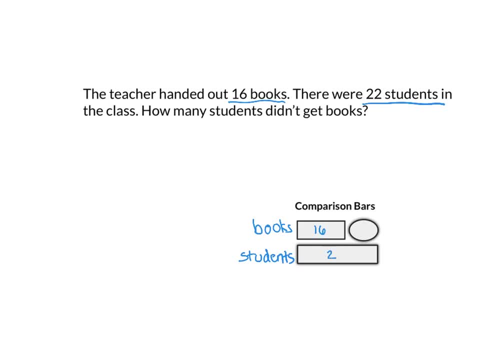 we also know the total number of students, that's 22.. so what we're trying to find out in this problem is the difference in the number of kids who didn't get books. so that's our question mark. so in this problem, because we have the total and we have um the number of books, we're trying 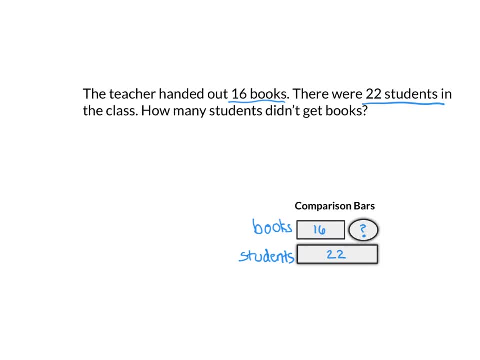 to find the difference. since we're trying to find that difference, it becomes a subtraction problem. so we can take our total, which is 22, and subtract the 16, and that'll give us our difference. i can't subtract 6 from 2, so i'm going to have to ungroup. 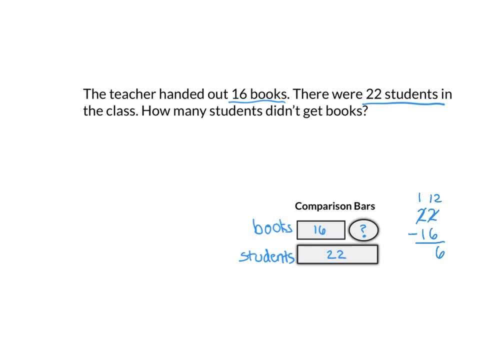 12 minus 6 is 6 and 1 minus 1 is nothing. so it looks like six students did not get books. let's look at one last problem. today, ethan had 17 pieces of candy. after he gave one to each of his siblings, he had 15 pieces left. how many siblings? that siblings does ethan have? 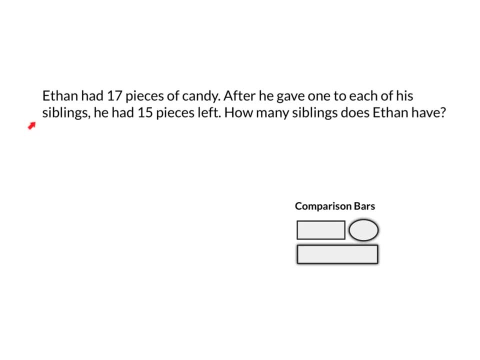 okay, we know he has 17 pieces of candy. he gave one to each of his siblings and then he had 15 pieces left. well, when, if he has 15 left, that has to be the difference. i'm going to right now write that in the difference. now, would he have more pieces of candy or more siblings? well, he had. 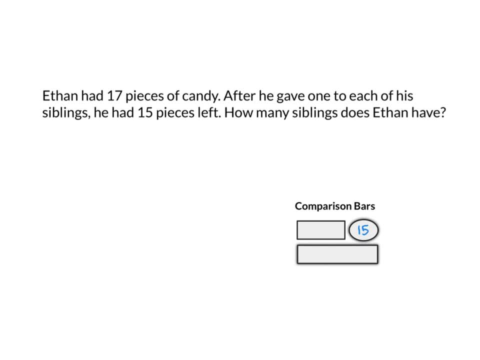 leftover candy. so there's no way that he has more siblings than candy. so i know that the siblings is going to be the smaller box and the candy is going to be the bigger box, and the problem tells us that he has 17 pieces of candy. so i can write that there and we're trying to find out how many. 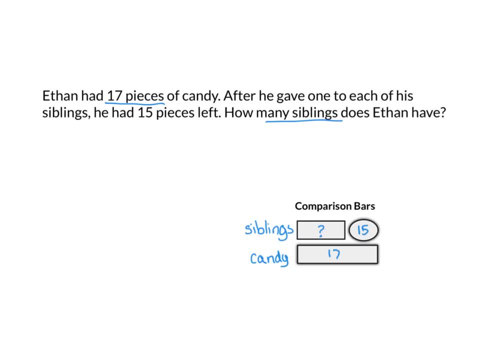 siblings he has. so that would be your question mark. so again, we have the total, our, we know our total, and then we have one of the top numbers is missing, so it's a subtraction problem. whenever we have that total filled out and we're missing one of the top two, it's a subtraction, so it's 17. 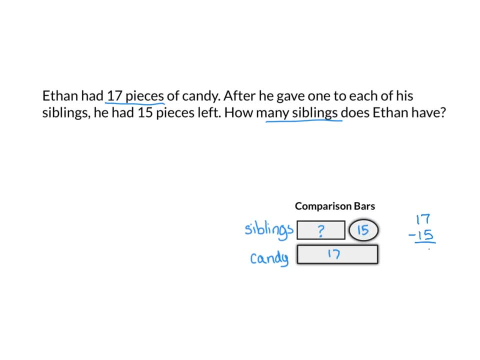 minus 15.. seven minus five is two. one minus one is nothing. so ethan must have two siblings, and i believe that is true. all right, that's it for today. i'll see you next time.